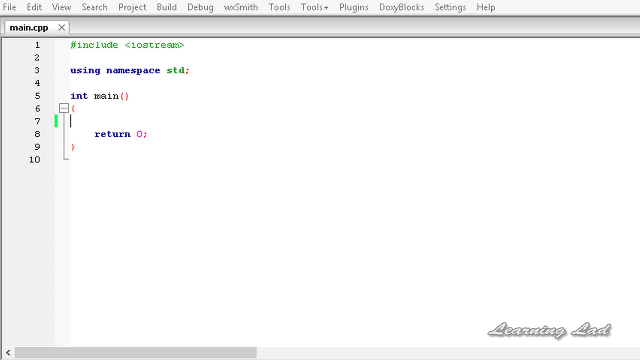 Hi, this is Sunil, and welcome to the video tutorial for the learning lab on C++ programming. So in this tutorial we gonna learn how to instantiate an object or create an object in different ways, and also how to access the members of a object using the arrow operator. 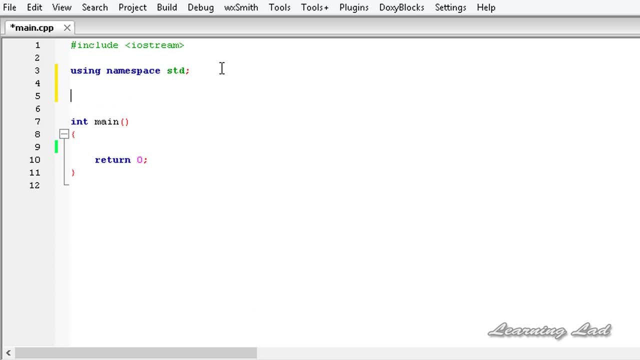 So here, just for the demonstration purpose, we gonna create a class before. our main function is gonna be class and let's say human and pair of curly braces, and between that curly braces we need to write the properties and methods of a class. So first we gonna write the access specifier, so it's gonna be public, and then let's create 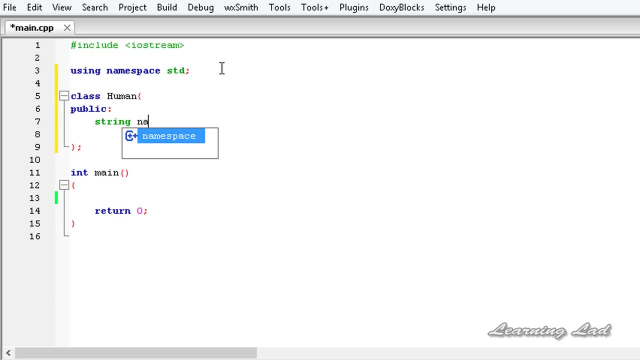 a property, let's call it as name and let's create a function called introduce. You know which we have done in the previous tutorial: the same thing. So this introduce is not gonna take any parameters and also not gonna return any values, and here in this introduce, we gonna write hi and then we gonna refer our name, and let's end this. 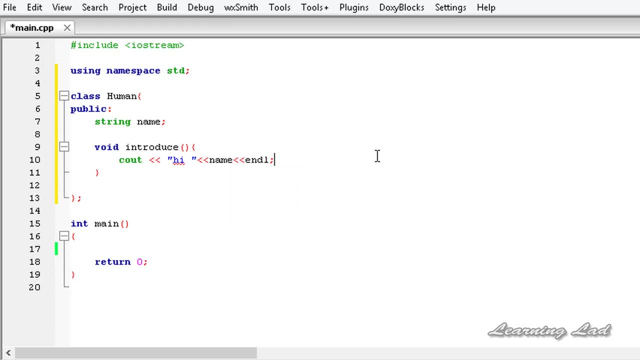 line. alright, Now we have a class definition or a class or the blueprint to create the objects. The next thing that we gonna do is we gonna create the objects in our program. So in the last tutorial, I have explained you how to create an object by specifying the. 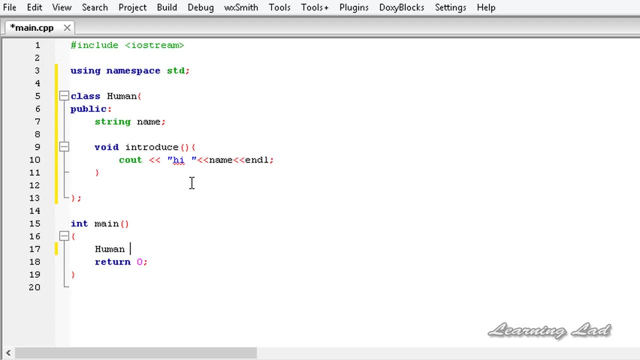 class name first- that is human- and then the name of the object, Let's say anil. So this is one type of creating an object from a class. So when you use this method, the object anil will be stored in the stack, not in the heap. 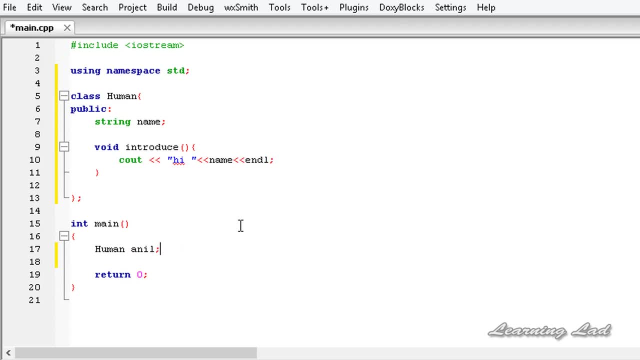 will be stored in the stack. The next way of instantiating an object is using this method. So in this method we gonna create an object. So in the last tutorial I have explained you how to create an object by specifying the class name using the new keyword. 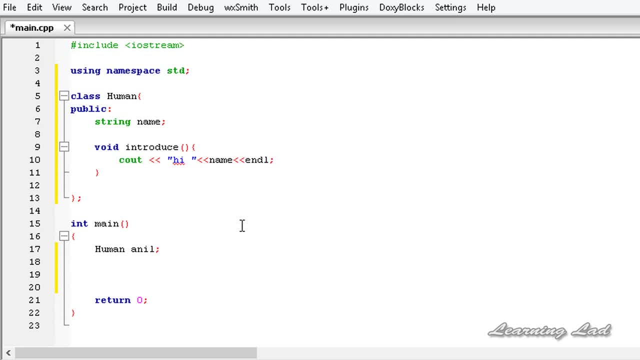 So when we use a new keyword, the object will be allocated in the heap and it will be dynamic, And also the new keyword is gonna return the address, memory address. that's why we need a pointer of this type: class human. So I'm gonna create human star. that's because it's a pointer. and then let's give a name. 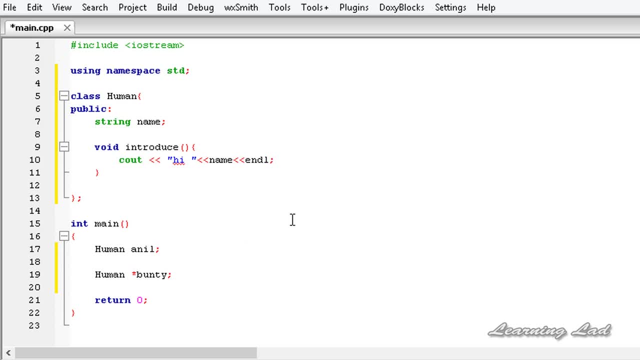 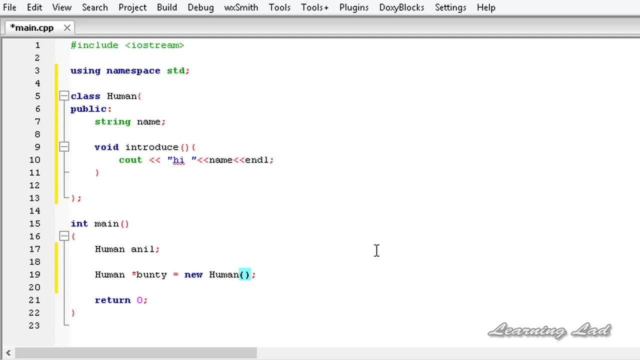 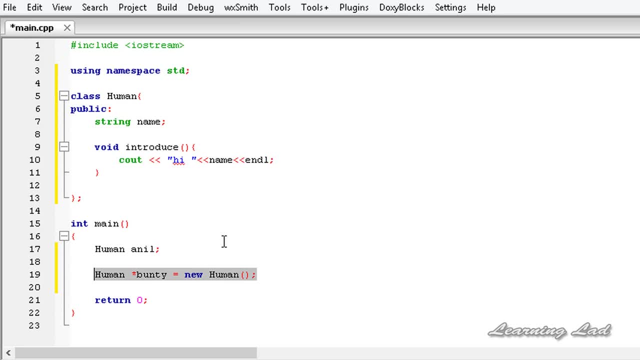 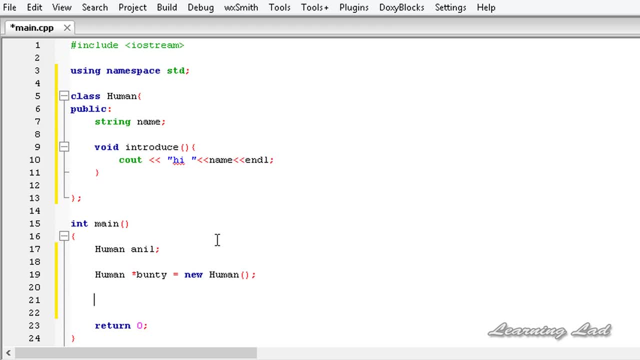 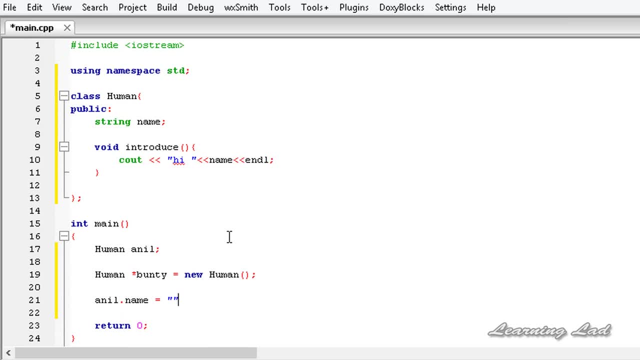 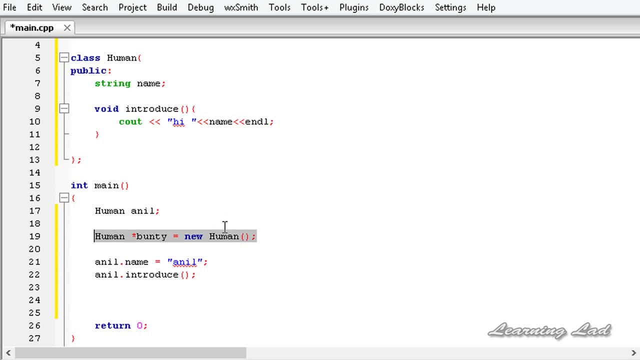 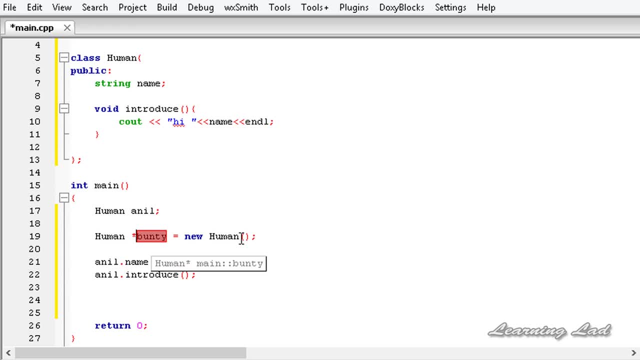 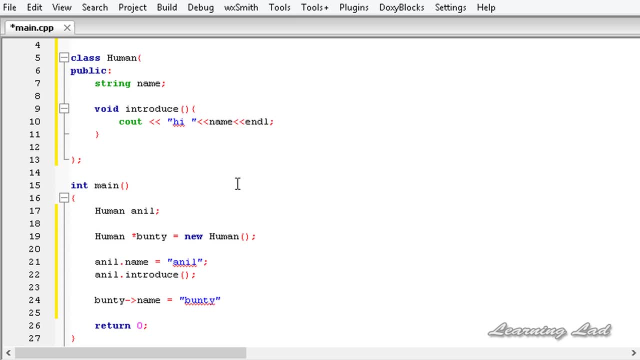 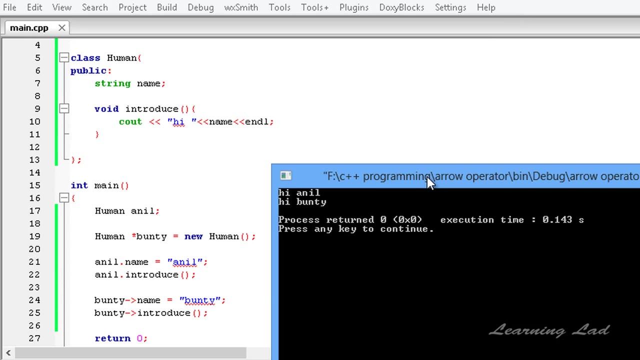 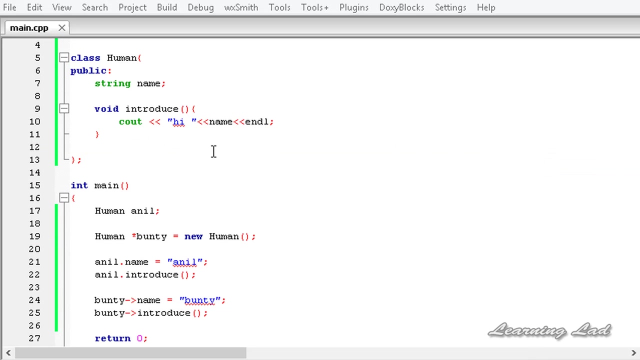 Bunty, Bunty, Bunty. we can call the method introduce by using the arrow operator in the same way. so bunty, arrow operator introduce, then add the semicolon. so i'm gonna save this, i'm gonna build and run this so you guys can see: here we got hi anil, hi bunty. so so in our programs we can create an object.